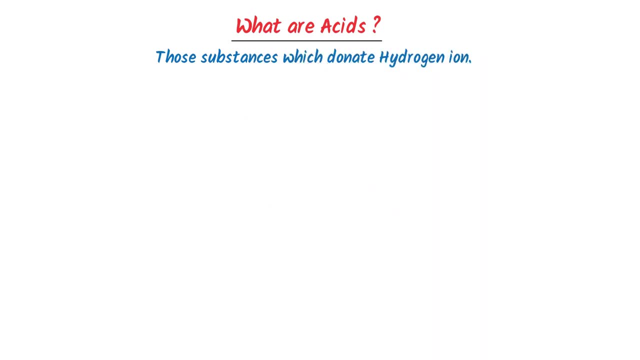 those substances which donate hydrogen ion are called acids. For example, consider hydrochloric. We know that hydrochloric can donate hydrogen ion, so we say that hydrochloric is an acid. Now how can we learn the list of famous acids? 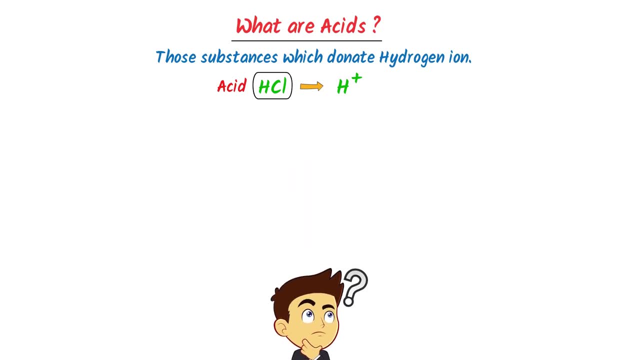 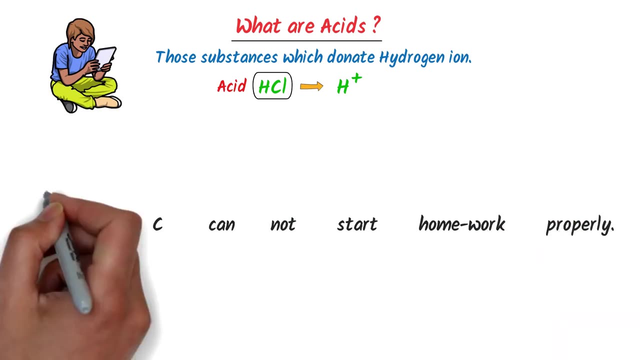 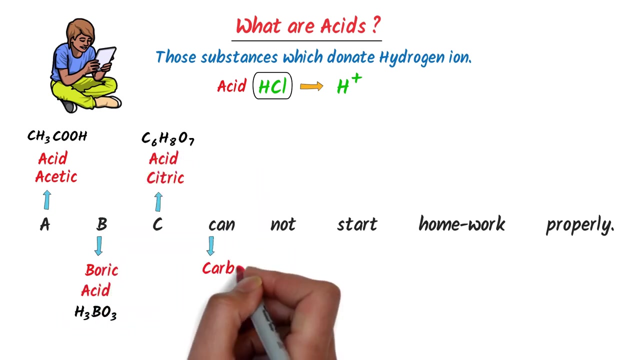 Well, to learn this, let me teach you my personal trick. I always say: ABC cannot start homework properly. Here, A stands for acetic acid, B stands for boric acid, C stands for citric acid. C stands for carbonic acid, N stands for nitric acid. 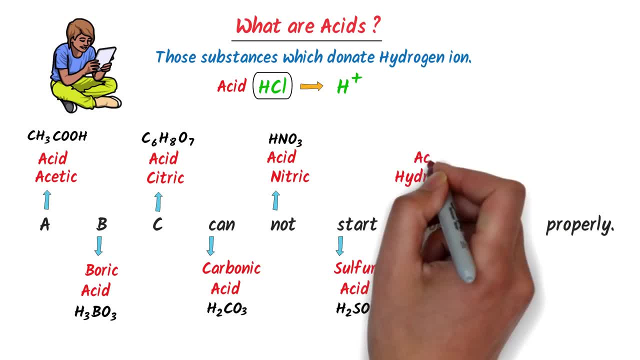 S stands for sulfuric acid, H stands for hydrochloric acid, P stands for phosphoric acid. So this is the list of all important acids which we study in the chemistry. Here let me teach you one important point: Remember that all these acids have hydrogen ions. So 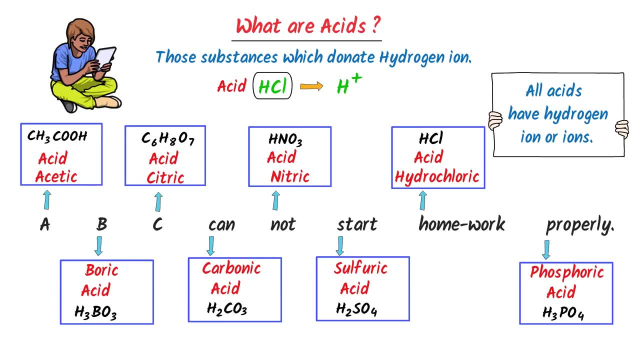 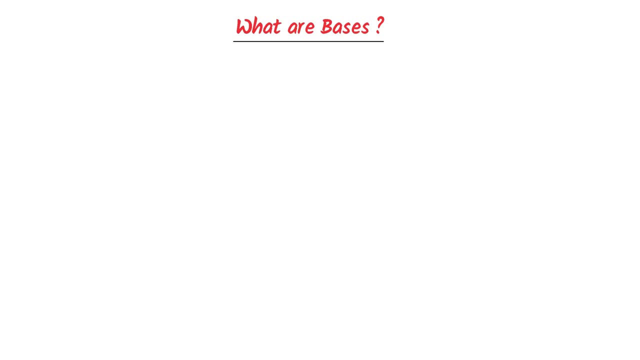 hydrogen ion is the best indicator of acid. Thus also noted down this important list of acids. The second main topic is: what are bases? Well, according to Arrhenius concept, those substances which can donate hydroxide ion are called bases. For example, consider sodium. 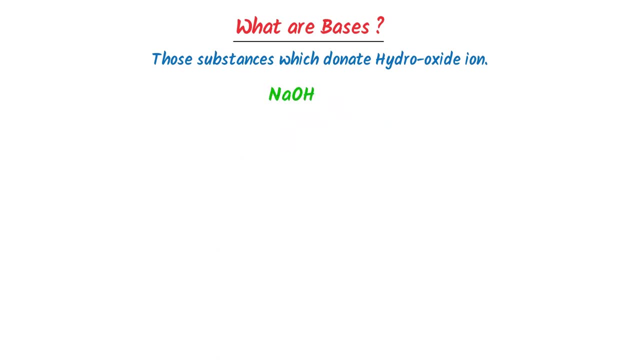 hydroxide. We know that sodium hydroxide can easily donate hydroxide ion, So we say that sodium hydroxide is a base. Now how can we learn the list of important bases? Well, I use my personal trick: I always write metals plus hydroxide ion always form bases. For example, consider group 1. 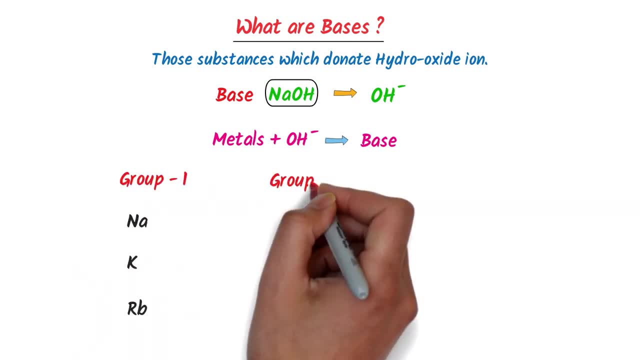 elements like sodium, potassium, rubidium. Consider group 2 elements like sodium, potassium and rubidium with a group of its enough volume than the number or coat And we will start the book with the group 2, elements like magnesium, calcium, and group 3 elements like iron, copper. 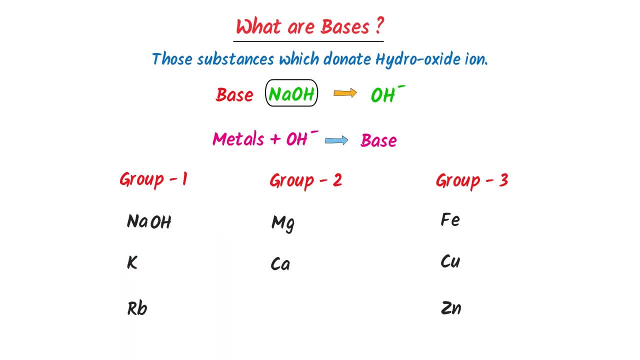 zinc. Now with group 1 elements, I write hydroxide ion like sodium hydroxide, potassium hydroxide and rubidium hydroxide. With group 6, I write 2-hydroxide ion like magnesium hydroxide. 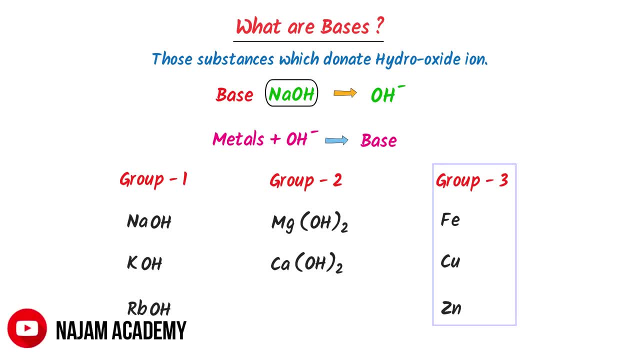 calcium Hydroxide, But you would also write co2 and co-, Cyrus and co2- and so forth. Here two hydroxide ions like iron hydroxide, copper hydroxide, zinc hydroxide. So all these metals containing hydroxide ions form important bases. 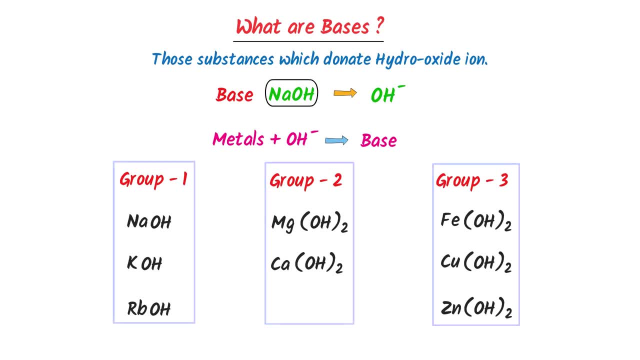 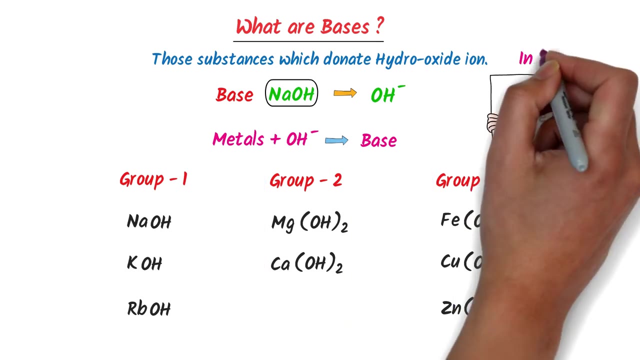 Thus, this is the list of all important bases Here. let me teach you one important point: Remember that all the bases have hydroxide ion. Let me repeat it: all the bases have hydroxide ion, So the hydroxide ion is the best indicator of bases. 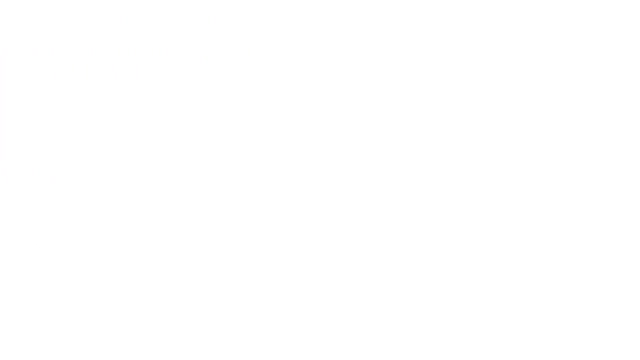 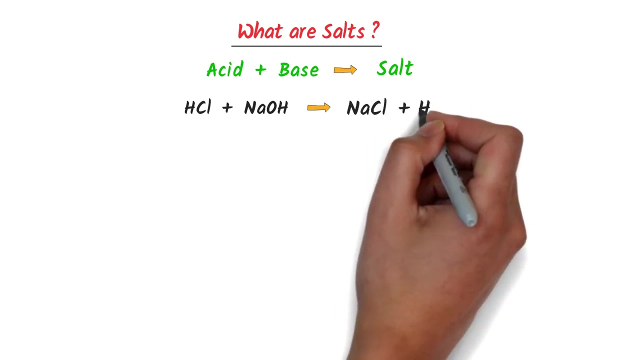 Thus noted down this important trick. Now, coming to the third topic, what are salts? Well, when acid plus bases react together, they form salt. For example, hydrogen chloride plus sodium hydroxide react together to form sodium chloride plus water. Remember that. 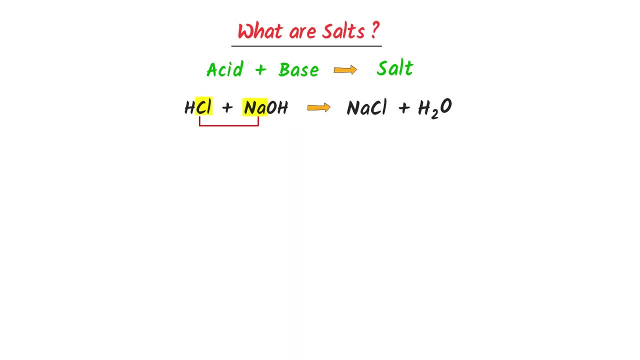 Here the metal part of the base, like sodium, and the negative part of acid, like chlorine. they will react together to form a salt, like sodium chloride, while the hydroxide ion of the base and the hydrogen ion of the acid would react together to form water. 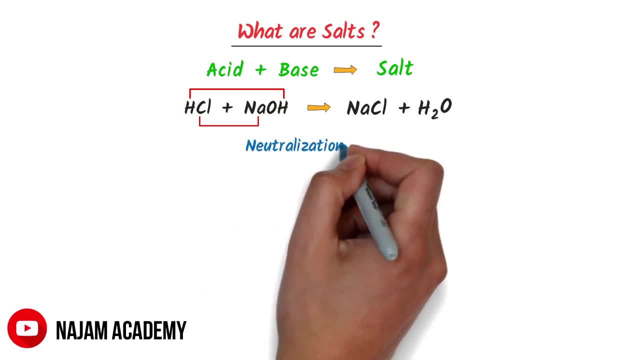 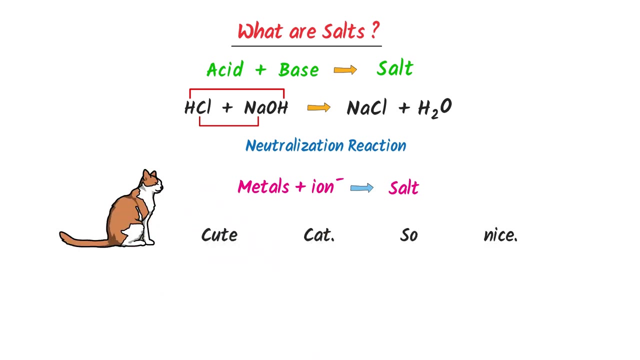 Remember that this whole reaction is known as neutralization reaction. Now how can we remember the important salts? Well, Needles full of metal plus ions usually form salts. Consider this cat. I always say that cute cat, so nice. C stands for chloride ion, like potassium chloride. 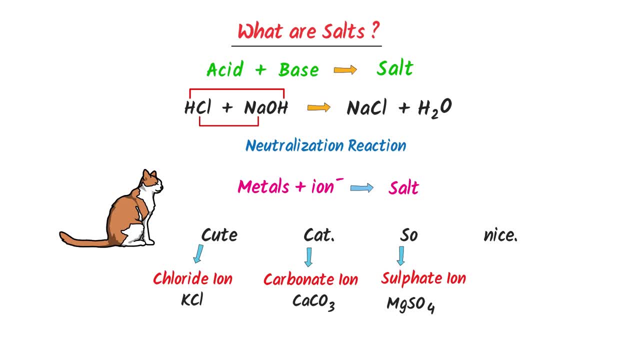 C stands for carbonate ions, like calcium carbonate S stands for sulfate ion, like magnesium. sulfate N stands for nitrate ion, like sodium nitrate. So if metal contains chloride ion, carbonate ion, sulfate ion or nitrate ion, then its trait ion- they are usually the salts. So remember this important trick about salts Also, let me teach. 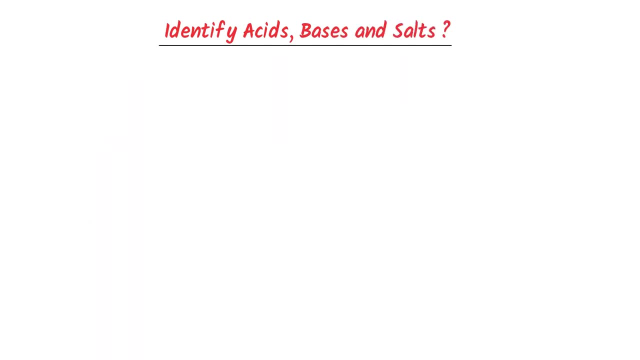 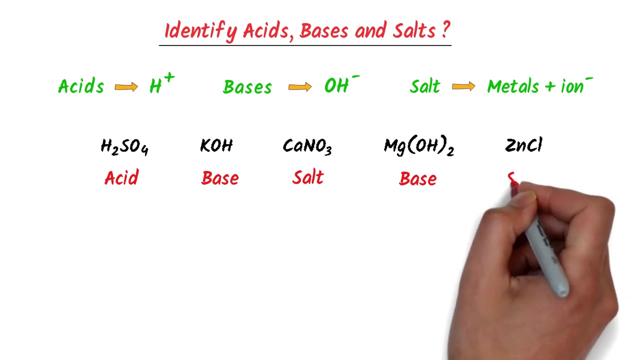 you one bonus question: How to identify acids, bases and salts? Well, consider this list. Now we know that acids contain hydrogen ion, base contain hydroxide ion and salt contains metals plus ions. So this is acid, this is base, this is salt, this is also base and this is salt. Thus, using this, 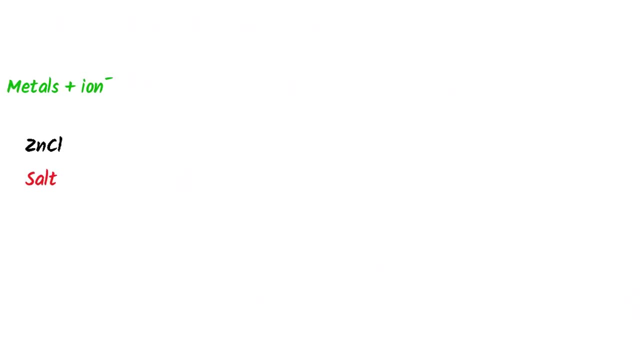 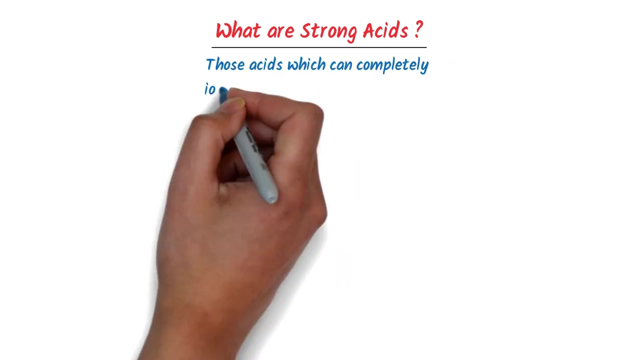 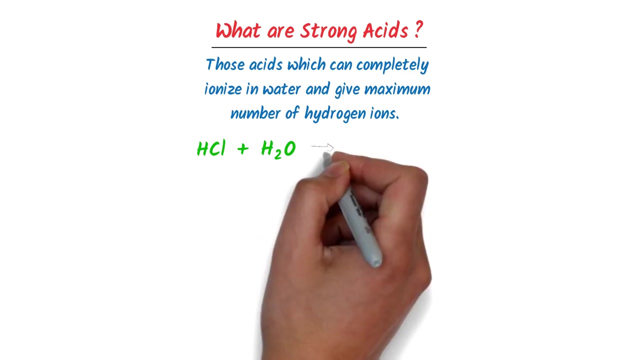 trick. we can easily identify acids, bases and salts. Now, what are strong acids? Well, strong acids are those acids which can completely desensuate our ionized and water and give maximum number of hydrogen ions. For example, consider hydrochloric acid plus water. We know that hydrochloric acid completely ionizes into hydrogen ion. 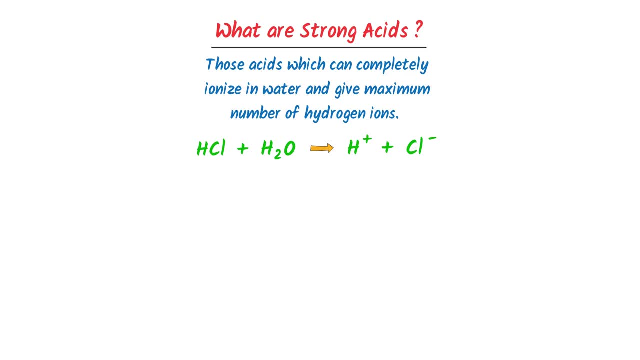 plus chlorine ion. So this is strong acid because it completely ionizes into hydrogen ion plus chlorine ion. Now how can we remember important strong acids? Well, I always say: not so hard. This N stands for nitric acid, HNO3, S stands for sulfuric acid, HNO4, HNO5, HNO6, HNO7, HNO8, HNO9,. 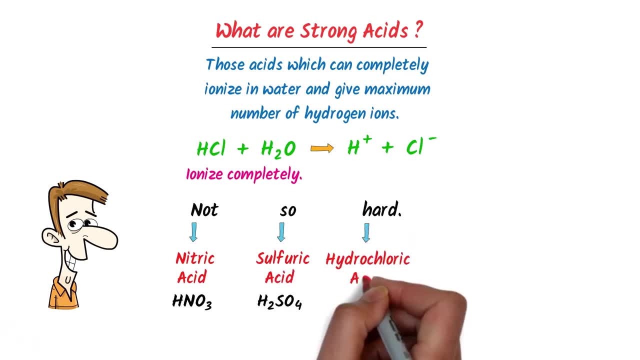 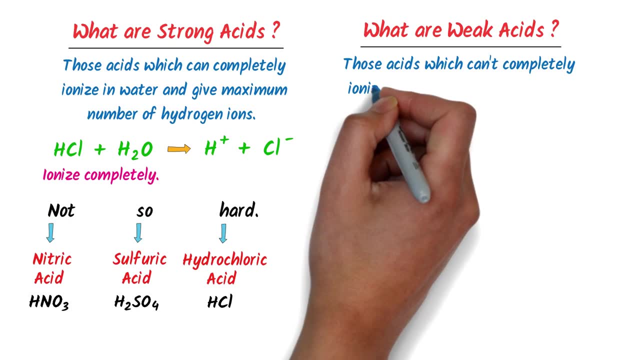 HNO8, HNO9, HNO12,, HNO3,, HNO6, HNO4, HNO7, and HNO8.. Now, how can we remember strong acids? Well, those acids which can completely desensuate our ionized and water and give lower number of 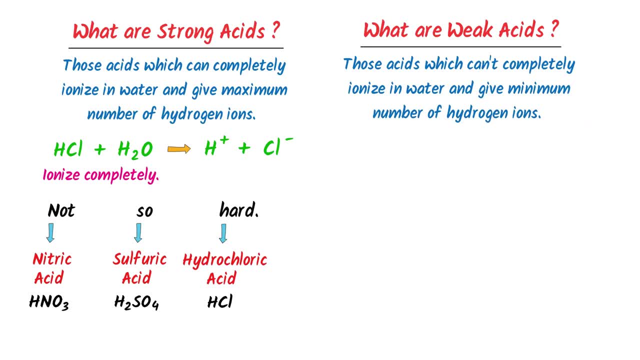 hydrogen ions. such acids are called weak acids. For example, consider acetic acid. When word dissolve acetic acid in water, it partially desensates in water. we can say that it can only ionize up to 1.3%, So it doesn't ionize completely in the water. 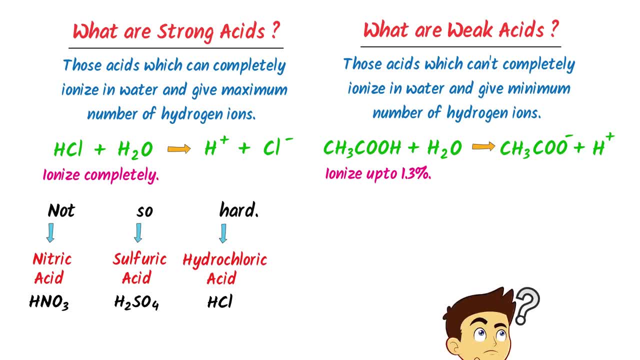 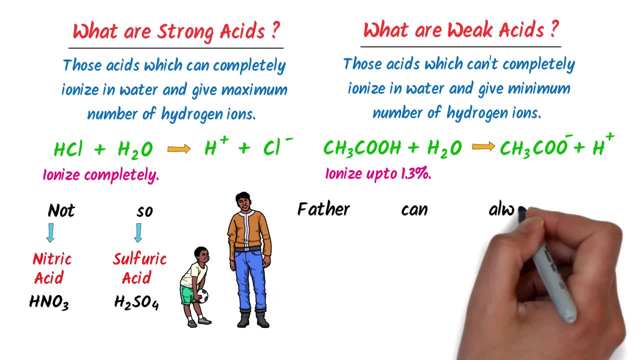 That's why we call it as a weak acid. Now, how can we remember the important list of weak acids? Well, I always use the trick: Father can always pay. F stands for formic acid, C stands for carbonic acid, A stands for acetic acid, P stands for phosphoric acid. So this is the list of weak. 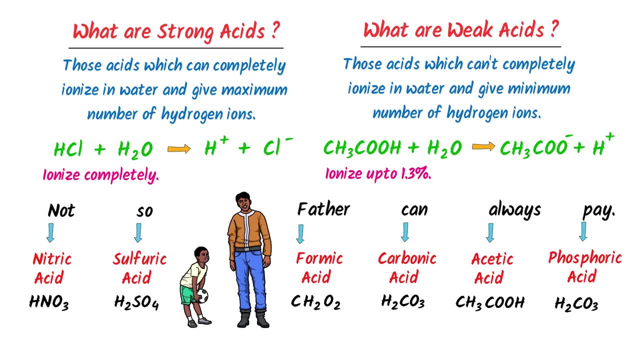 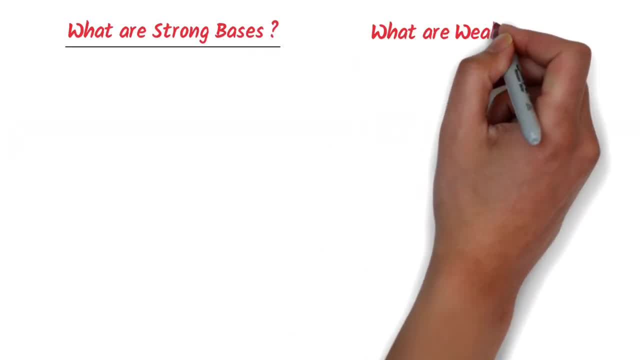 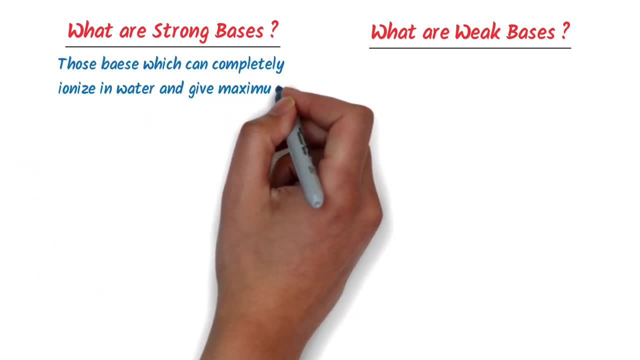 acids. Remember that we have already learned about the concept of strong species and weak species. Now we can easily learn strong bases and weak bases. Remember that strong bases are those bases which can completely ionize in water and give maximum number of hydroxide ion. 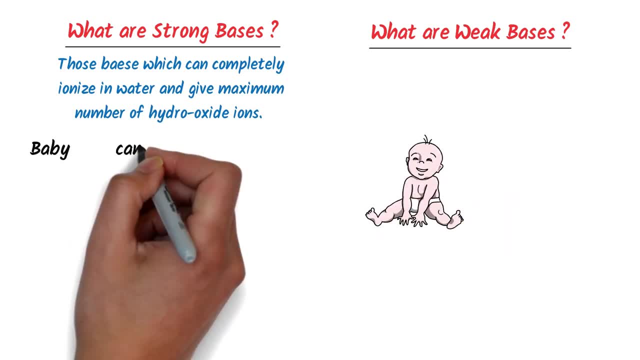 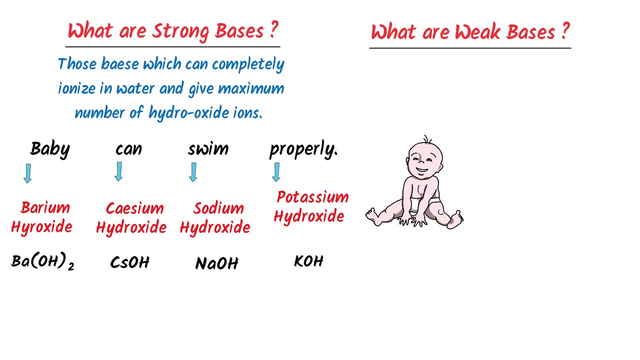 The trick to remember. the list of strong bases are- baby can swim properly. B stands for barium hydroxide, C stands for cesium hydroxide, S stands for sodium hydroxide, P stands for potassium hydroxide. So this is the list of strong bases. On the other hand, those bases, 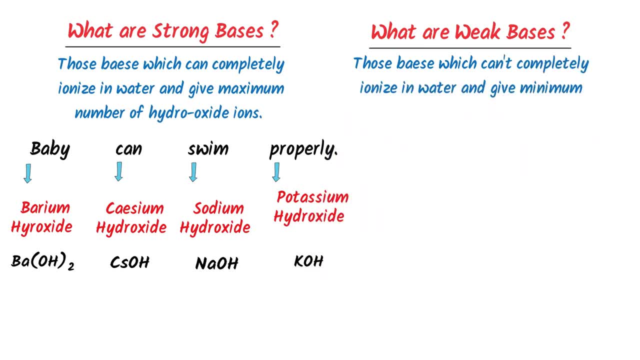 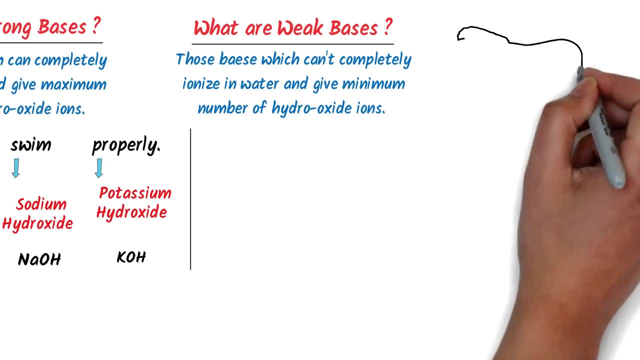 which cannot completely dissociate, are ionized in water and give lower number of hydroxide ion than the weak acids. So this is the list of strong bases. The trick to remember the list of weak bases are: can I always love zebra? Here C stands for 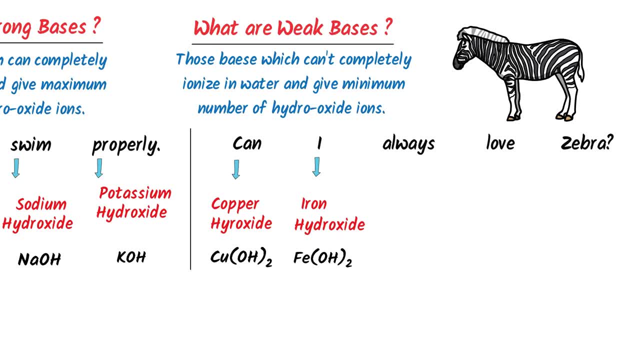 copper hydroxide, I stands for iron hydroxide, A stands for ammonia, L stands for lead hydroxide and Z stands for zinc hydroxide. So this is the list of important weak bases. So note it down, these important points. 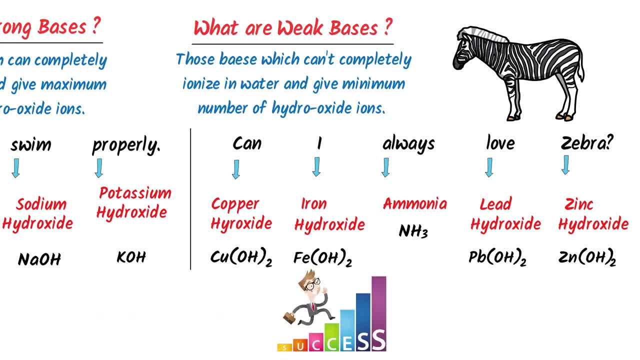 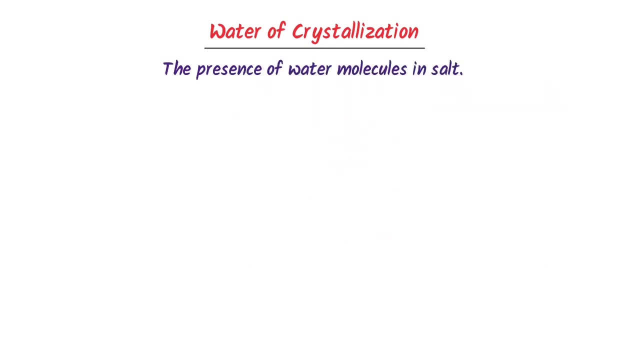 Remember that I will skip some very easy topics like indicator pH scale, importance of pH scale, which we have already learned in primary school. Now we will learn about water of crystallization. Well, the presence of water molecules and salt is called water of crystallization. 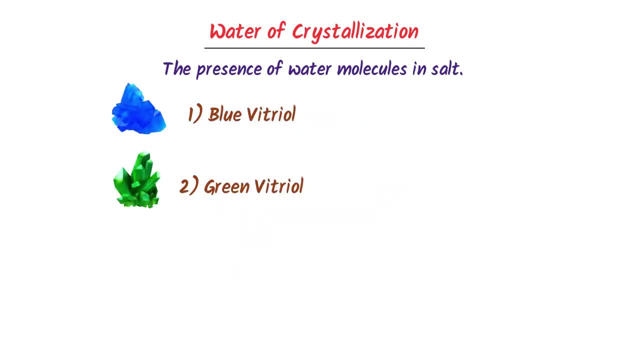 For example, like blue vitriol, green vitriol, white vitriol, Blue vitriol is copper sulfate, which contains 5 molecules of water. Green vitriol is iron sulfate, which contains 7 molecules of water. 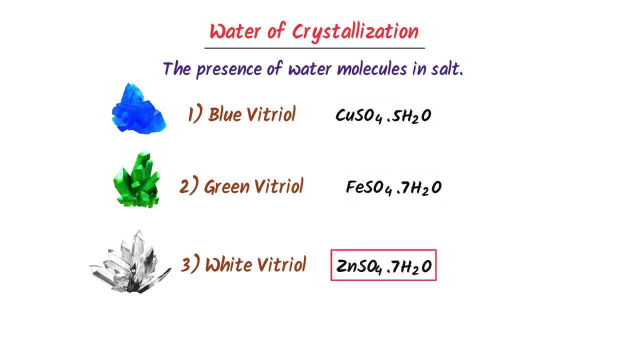 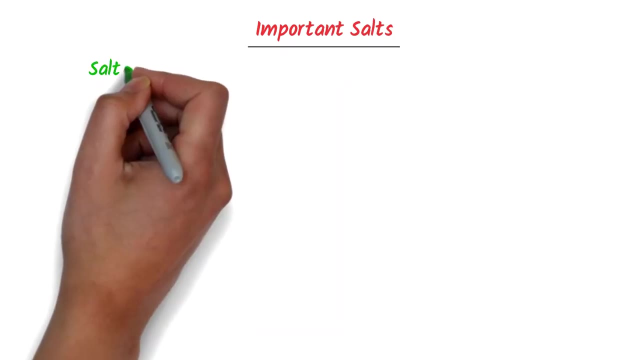 White vitriol is zinc sulfate, which also contains 7 molecules of water. So remember that water of crystallization is the salts which contain molecules of water. Lastly, let me teach you some important salts: their name, common name and uses. 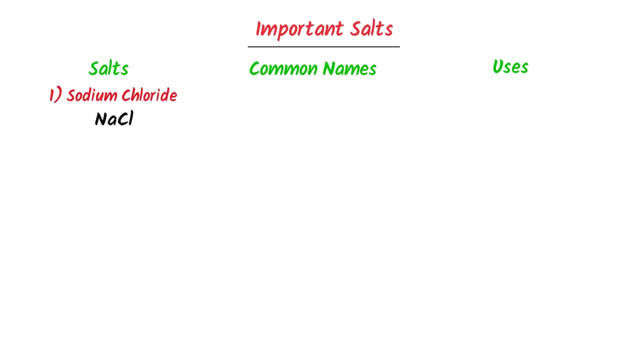 The first important salt is sodium chloride. The common name of sodium chloride is common salt. In daily life we use sodium chloride for seasoning purpose and in different food. The second important salt is calcium carbonate. The common name of calcium carbonate is limestone and it is used in construction of building.